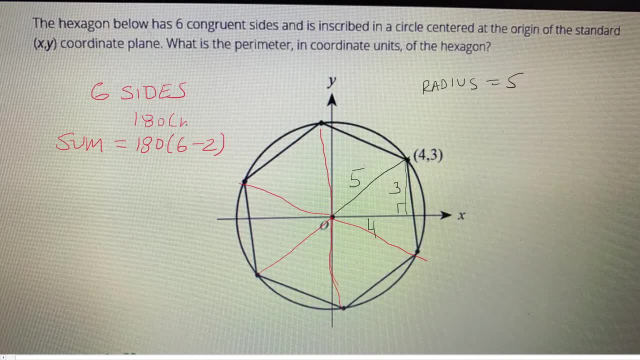 minus 2.. So the formula in general is 180 times n minus 2.. But here n is 6 because we have six sides. So that's 180 times 4, which is 720.. And now we're going to divide that by how many angles there are. So there's. 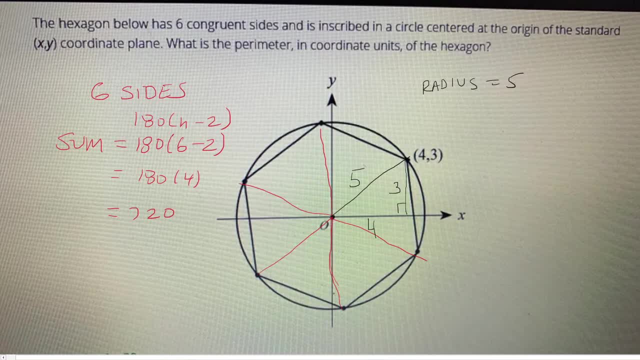 1, 2, 3, 4, 5, 6, 7, 8, 9, 10, 11, 12.. So there's 12 basically angles here. So 720 divided by 12. That's going to be 60. So that means we're going to have a hexagon. 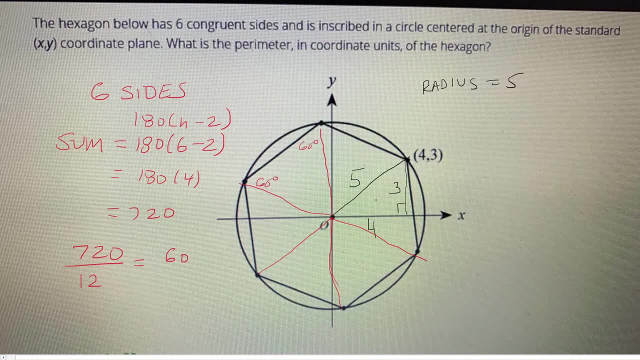 So that means we're going to have a hexagon. So that means we're going to have a hexagon. So that means each one of these guys is 60 degrees Etc. And obviously let's just take this triangle. here The angles have to add up to 180.. So so far you have 60 and 60 is. 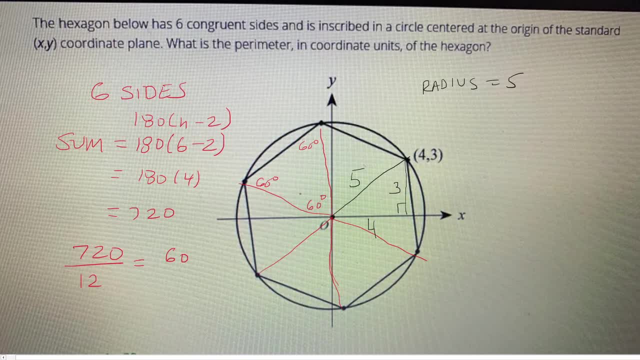 120. So we need another 60 to make 180.. So when the angles are congruent, this is where you get an equilateral triangle. So we show that the sides here are 5. And so that means we have a hexagon. So that means we're going to have a hexagon, So that means we're. 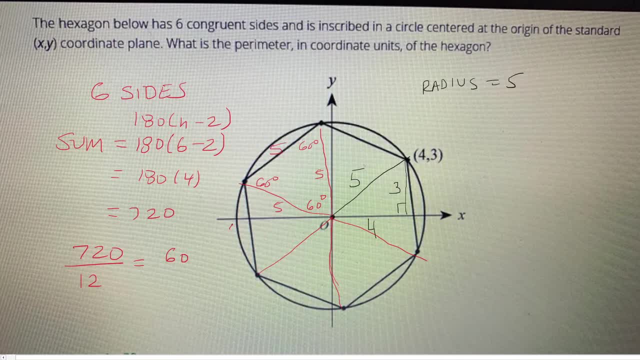 this side is also five, so we can just put fives around here, and so the perimeter it's going to be five times six, which is thirty. 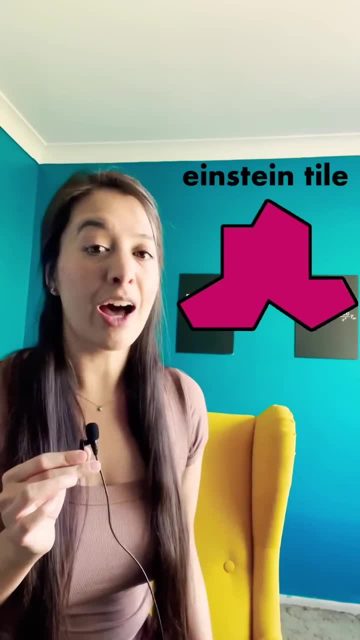 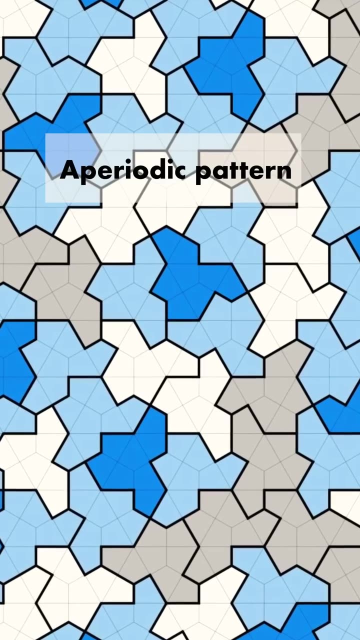 Guys, there's been a breakthrough in mathematics over this new shape. It's called an Einstein tile, meaning one stone, and it's the first ever single aperiodic tile ever discovered. An aperiodic pattern is one that can cover an entire surface without gaps and without 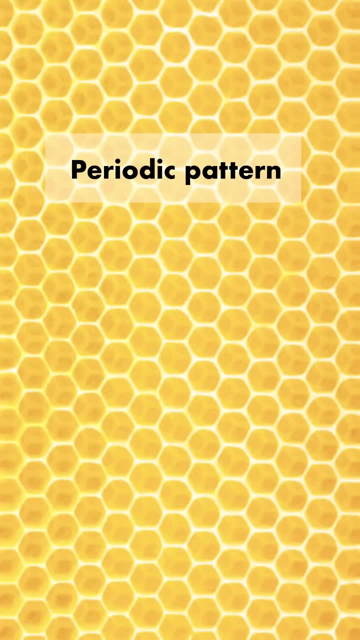 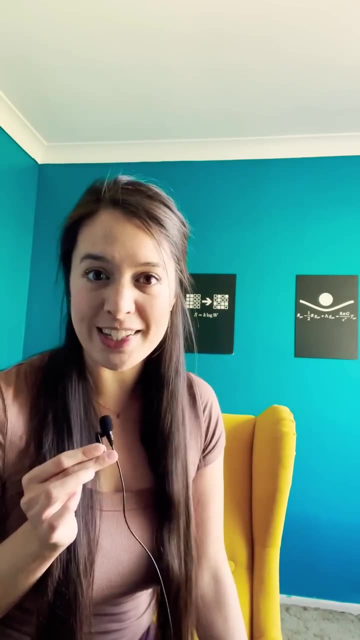 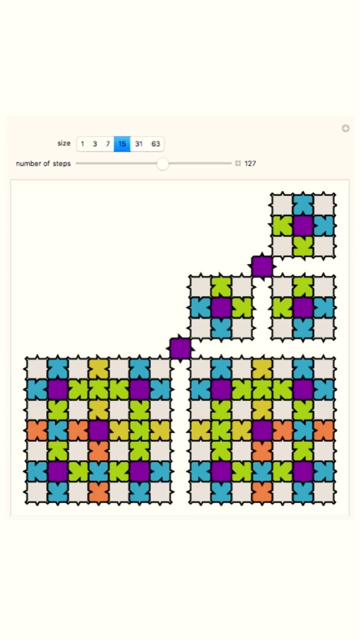 creating a repeating pattern. Compare this to periodic patterns, which are created by repeating a small cluster of shapes over and over again. Mathematicians have been fascinated by aperiodic patterns for centuries. In 1968, the computer scientist Donald Knuth found an example with 92 tiles. Then mathematician Raphael Robinson.